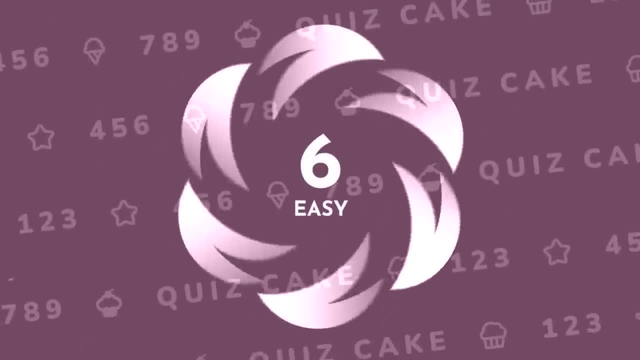 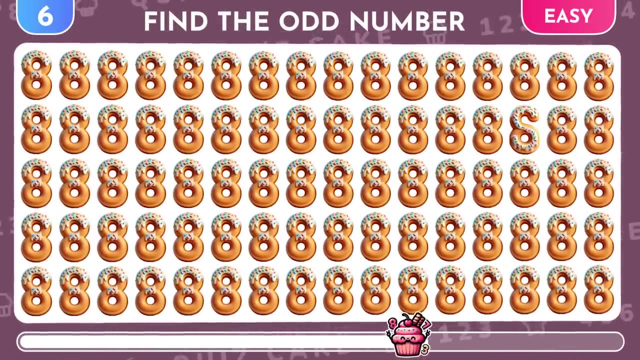 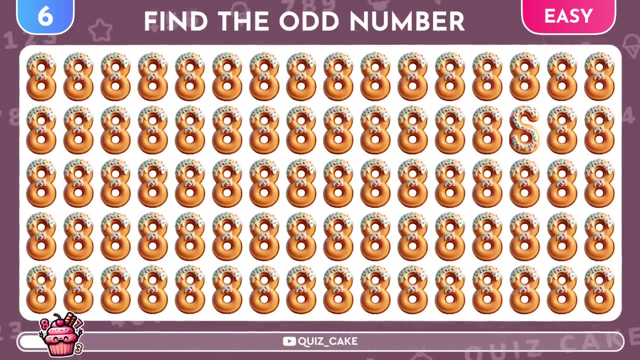 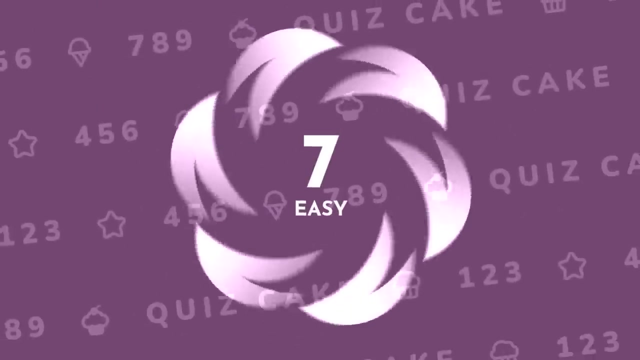 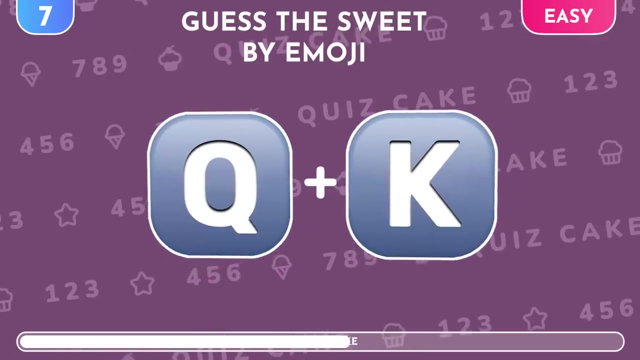 It's the number eight. It's the number eight. Now, It's the number eight. It's the number eight. Among these eights, there's a rebel digit. Can you identify it? Yes, it's the number six. Emoji challenge time. Guess the sweet treat from these two emojis. 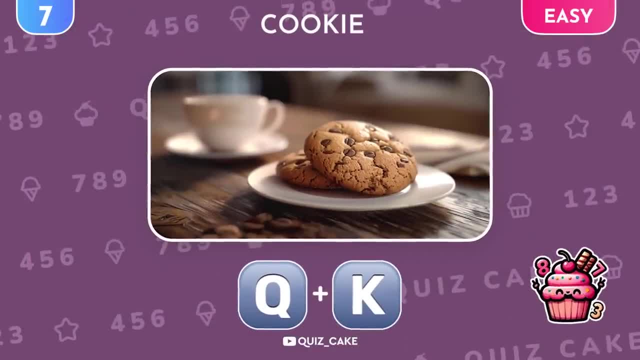 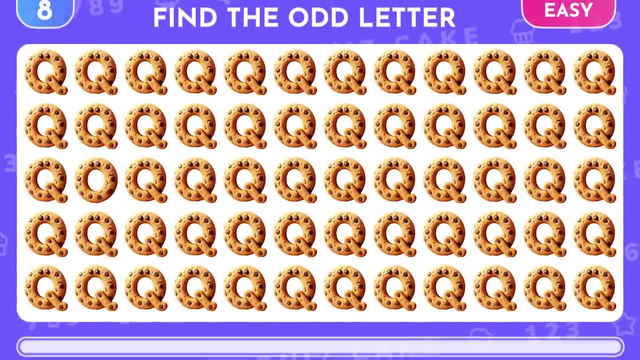 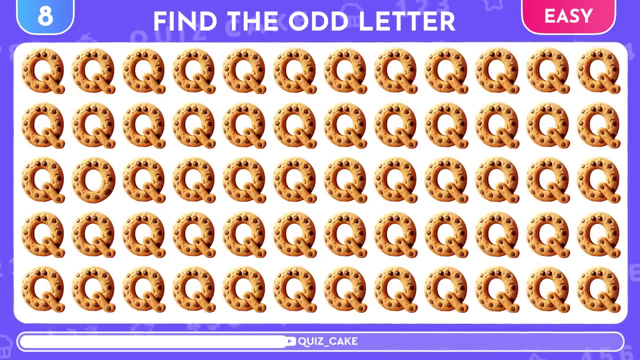 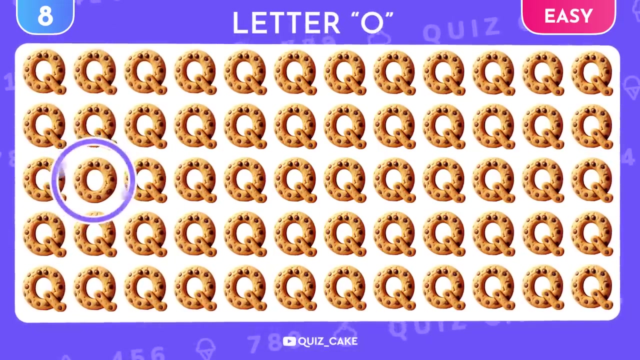 Emoji challenge time- Guess the sweet treat from these two emojis. The sounds Q and K come together to spell cookie. Emoji challenge time- Guess the sweet treat from these two emojis. Time to spot the odd letter out again. Emoji challenge time- Guess the sweet treat from these two emojis. 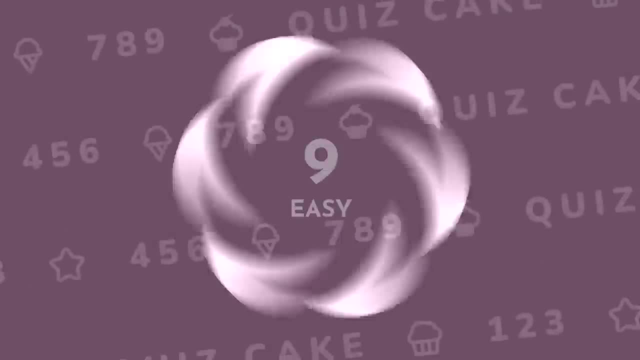 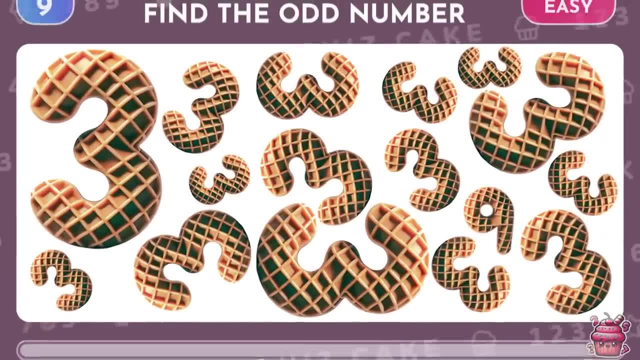 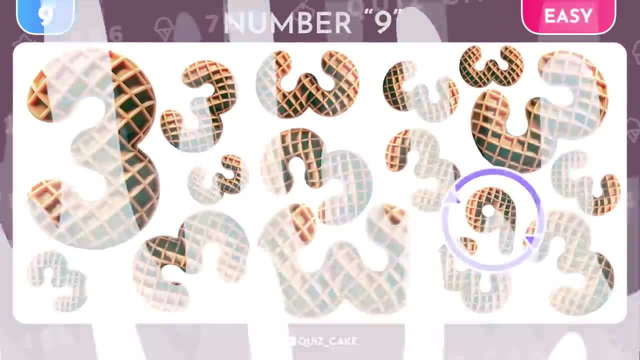 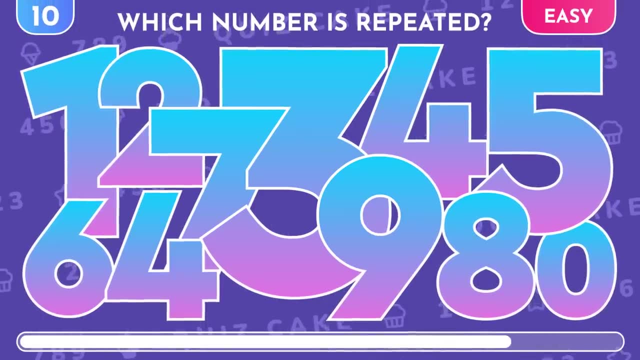 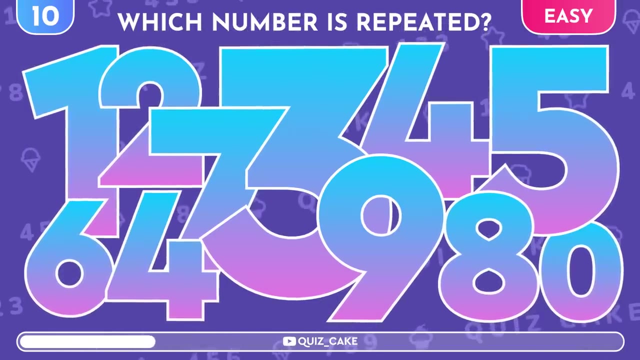 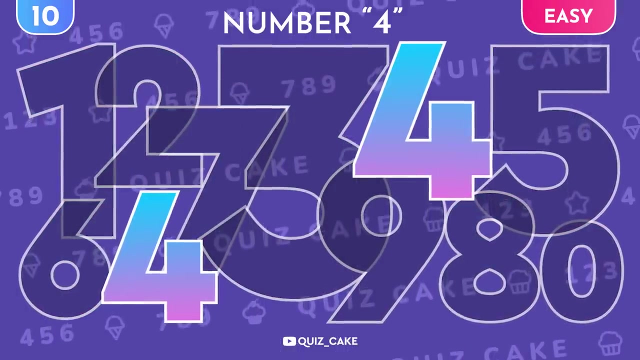 Yes, it's the number 9.. Now pay extra attention. Find the number that appears twice. The correct answer is 4.. This number shows up twice. Let's ramp up the difficulty to medium level. Find the letter that doesn't belong. 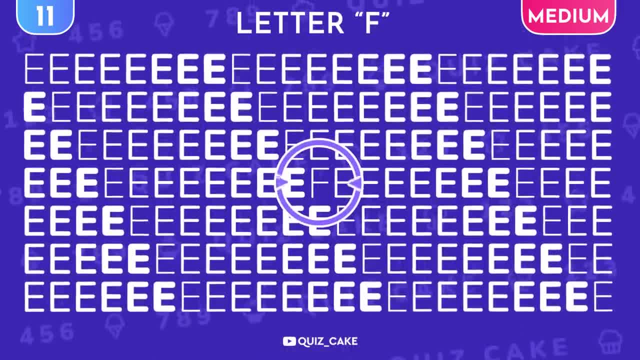 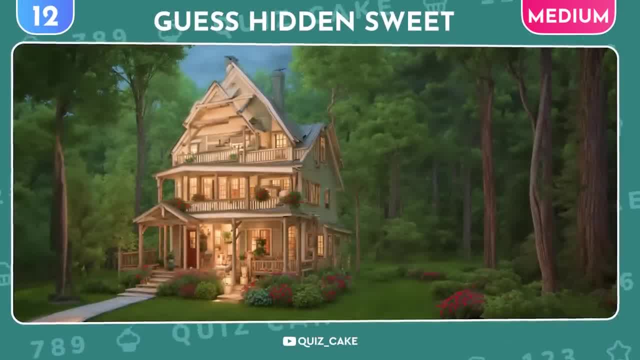 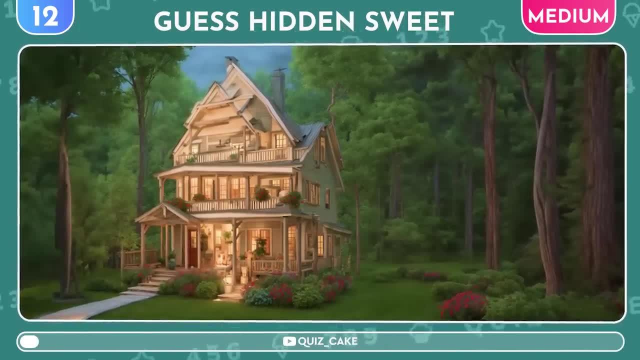 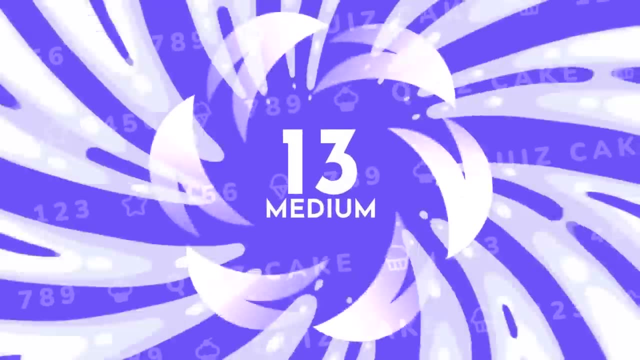 Awesome, It's the letter 9.. Find the letter F right in the center. Illusion time. Can you guess the sweet treat camouflaged in this picture? Wow, It's an ice cream. Try finding the kitty among a sea of ice creams. 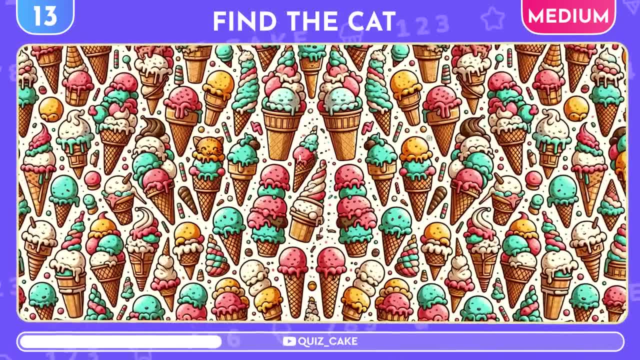 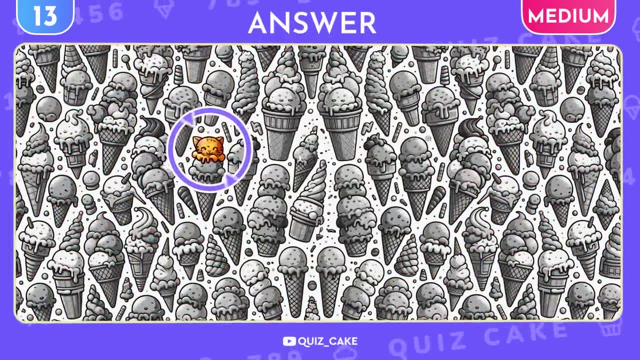 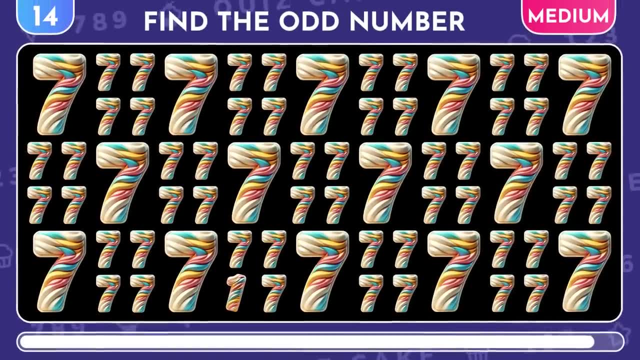 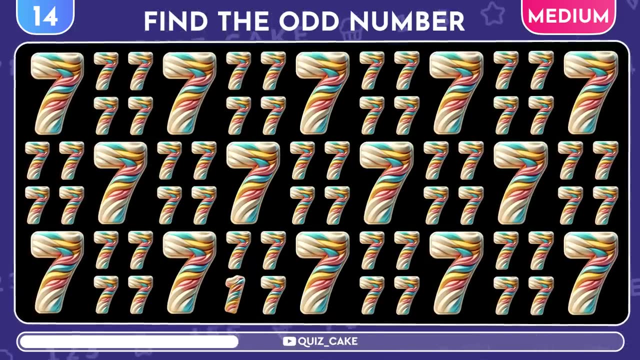 There's the kitty Right here among the sweets. To find the kitty among a sea of sweet treats. Identify the different digit. There's the kitty Right here among the sweets. Identify the different digit. The correct answer is 4.. Didn't we find the kitty? 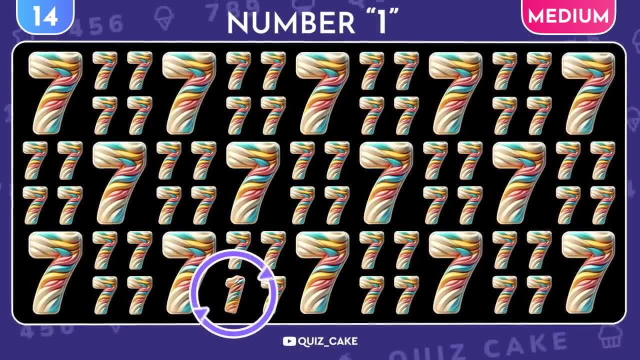 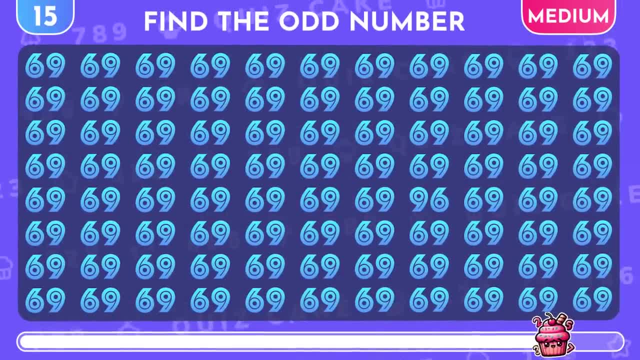 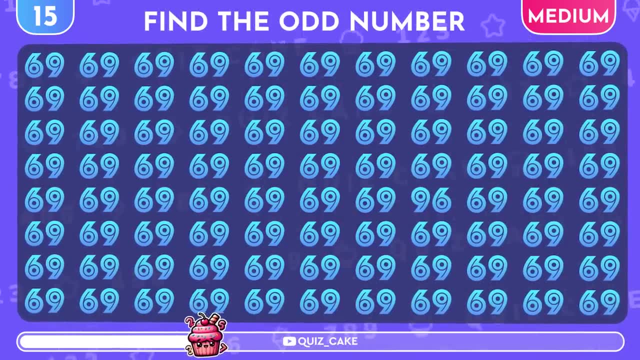 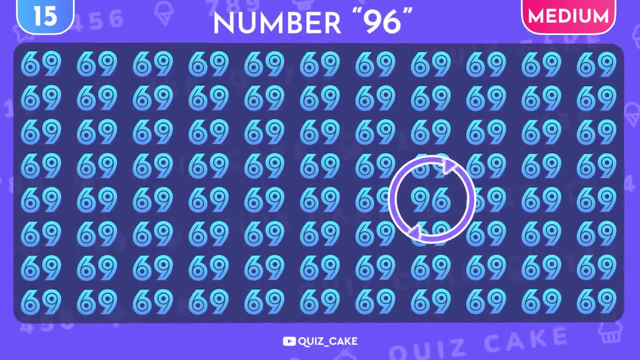 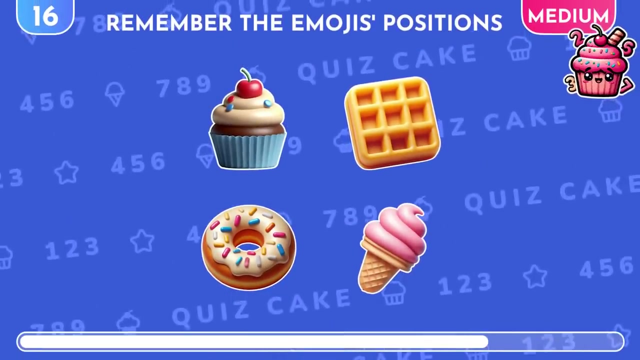 Yeah, Nice. So how about this one? Correct, it's the number 1.. How about this one? Can you spot the odd number out? Superb, it's the number 96.. Check your photographic memory. memorize the position of all 4 emojis. 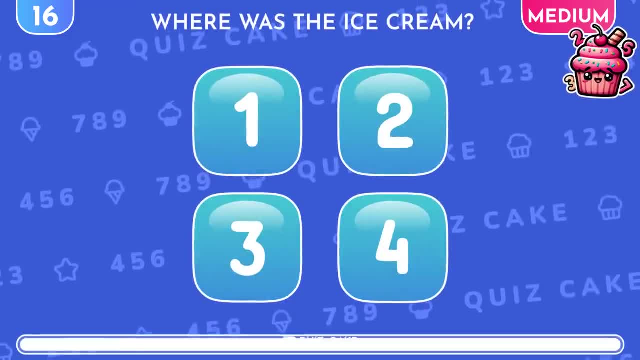 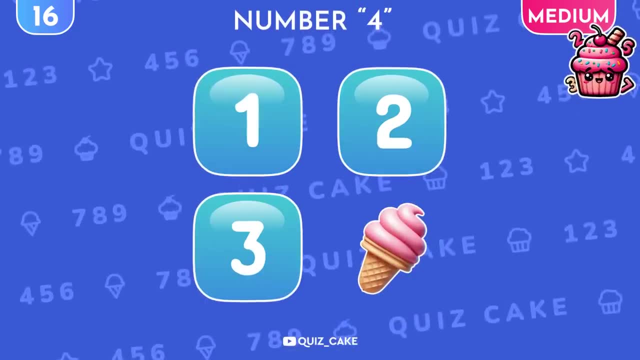 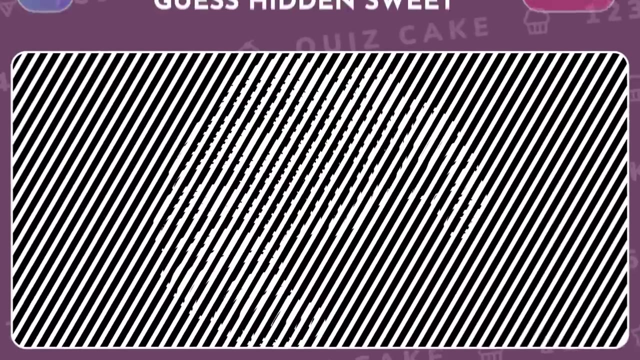 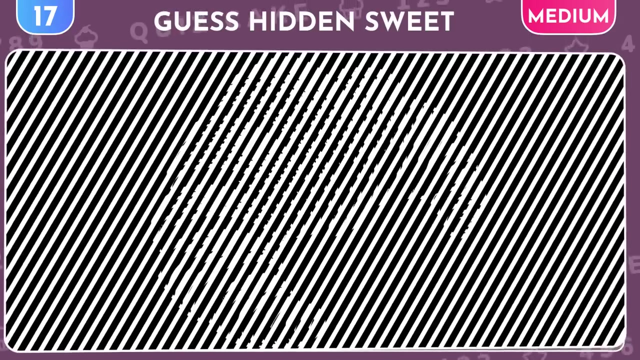 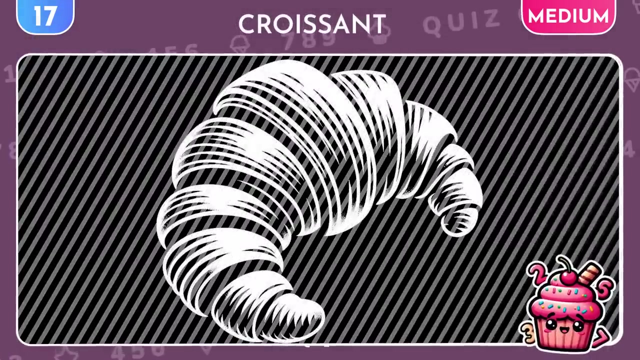 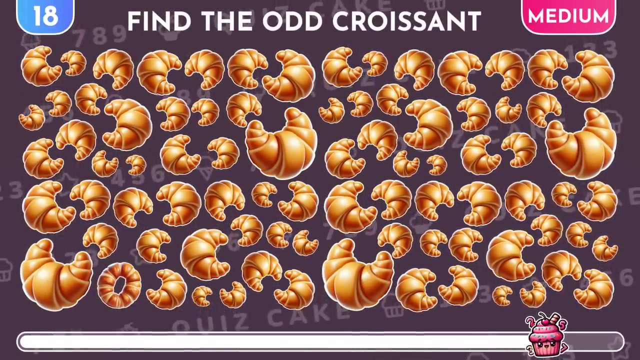 Ready, Now recall where the ice cream was. The ice cream was hiding under number 4.. Another optical illusion. What sweet treat does it conceal? Oh, It's a croissant. Well done, Now try to find the unique croissant emoji. 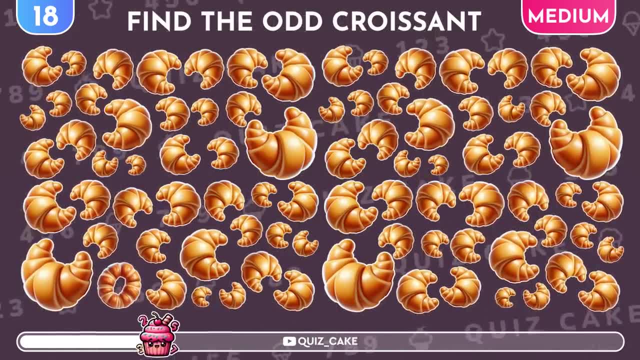 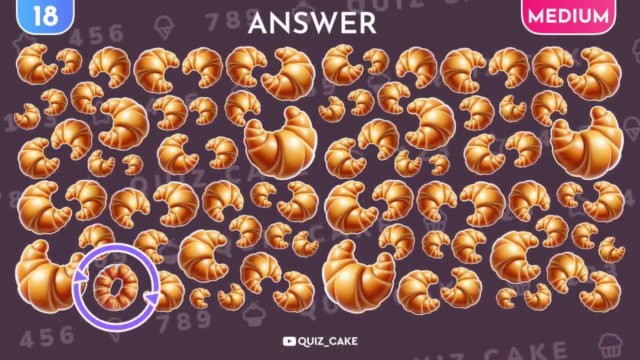 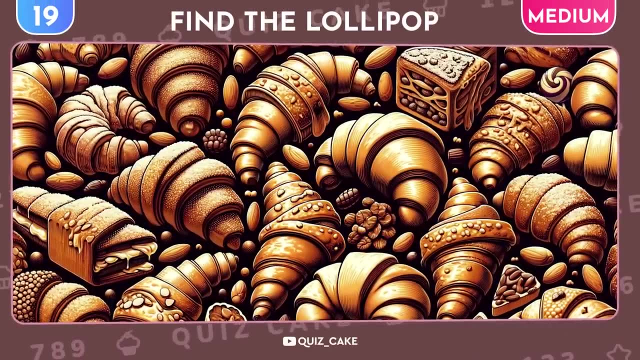 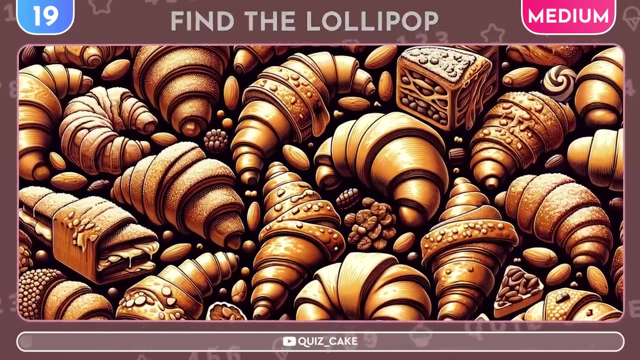 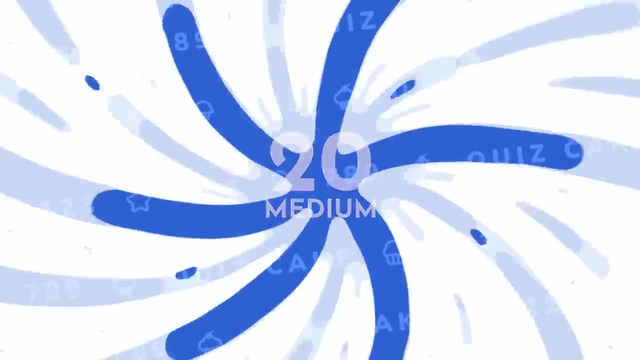 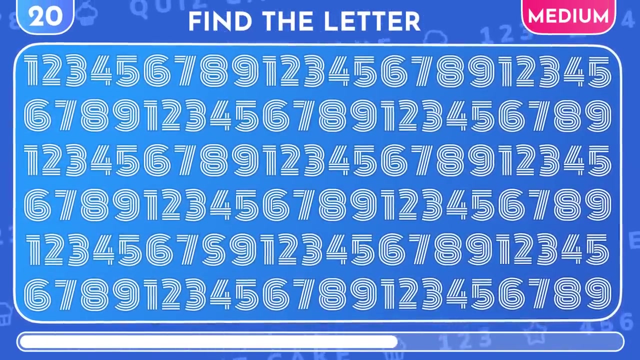 Wow, This croissant is round. Find the lollipop among the croissants. There it is, in the right corner, Among these numbers, hides a letter. Can you find it? It's a letter. It's a letter, It's a letter. 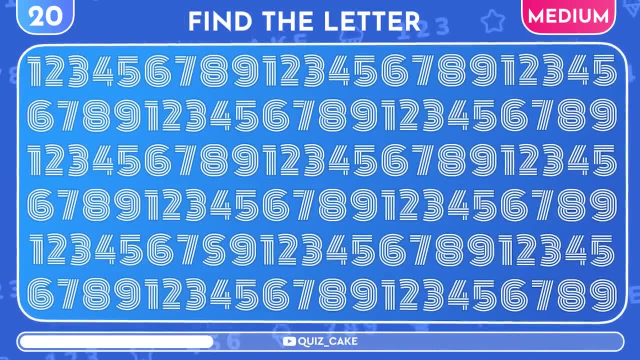 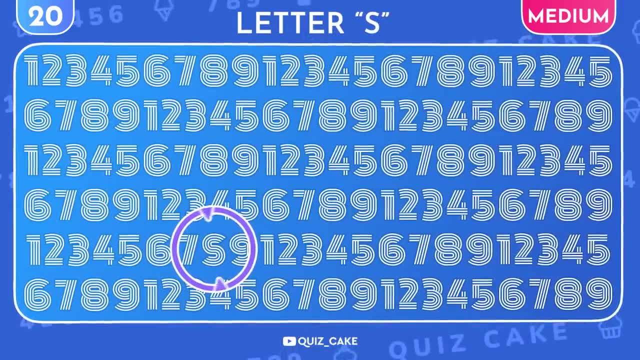 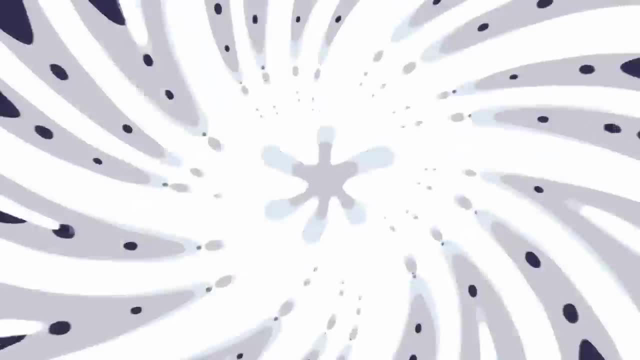 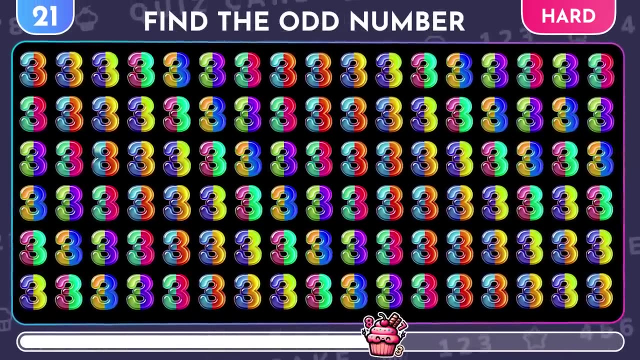 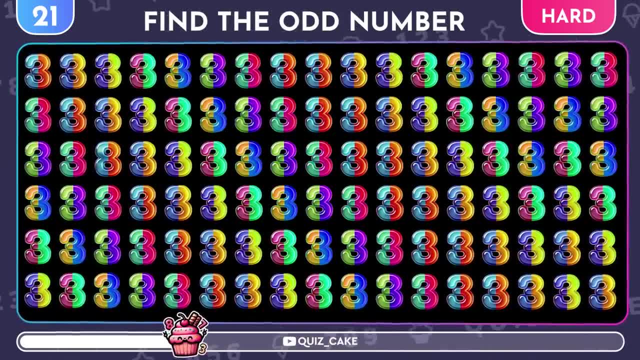 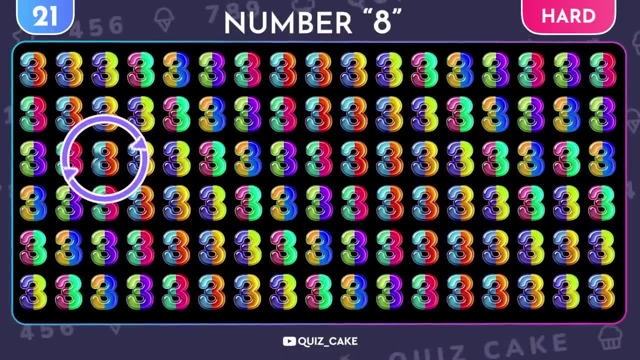 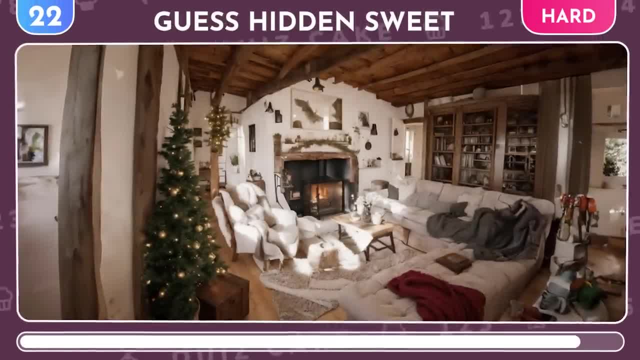 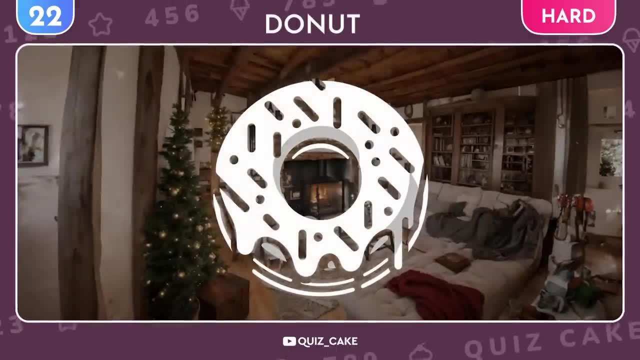 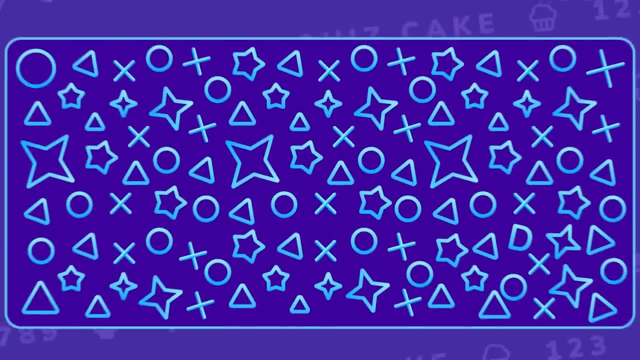 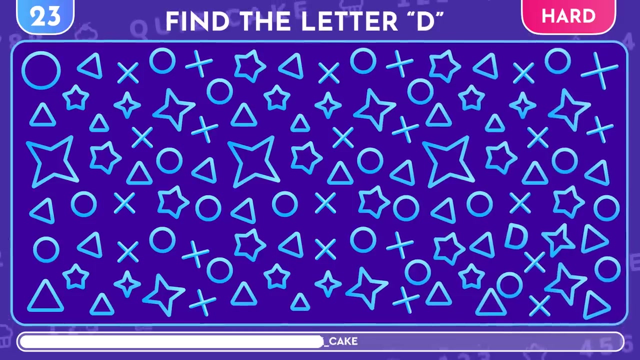 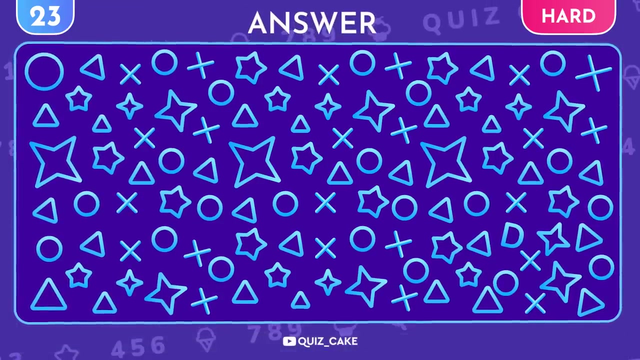 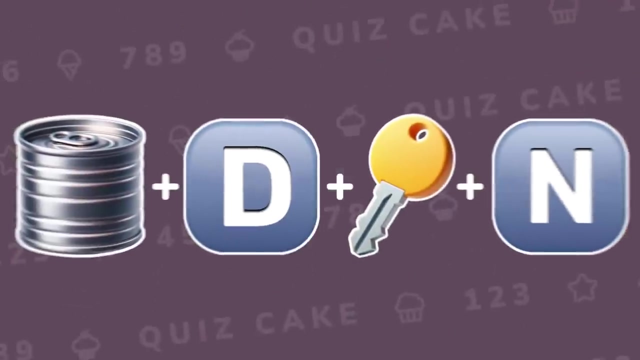 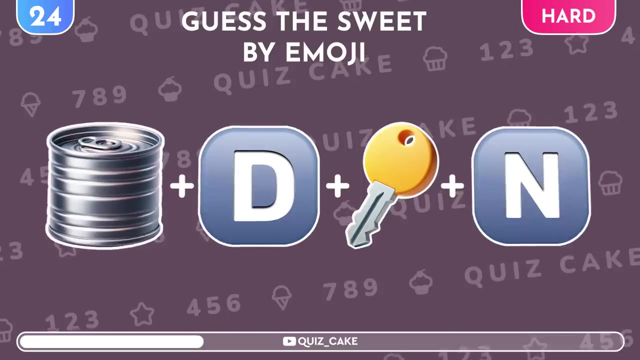 Guess the sweet treat hidden in this cozy room. Of course it's a sweet donut. Now try to find the letter D among these shapes. There it is Right here. Guess the sweet treat from these four emojis. Oh, It's candy cane. 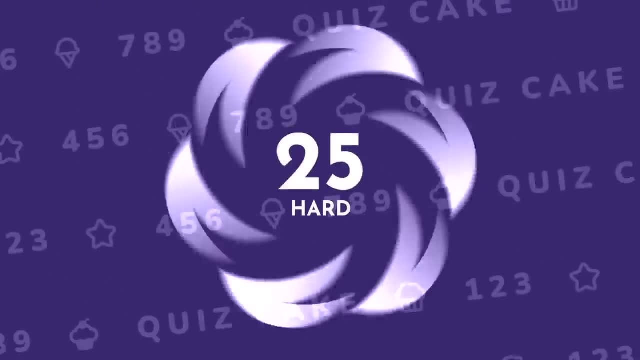 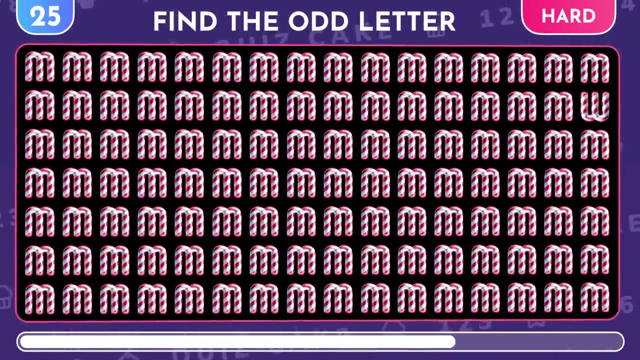 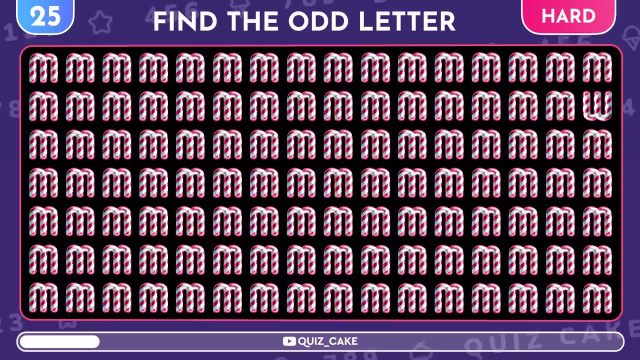 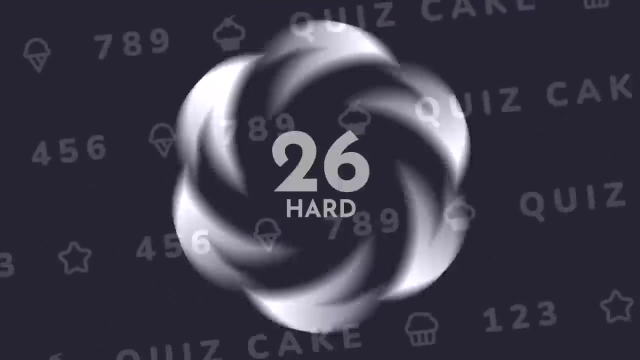 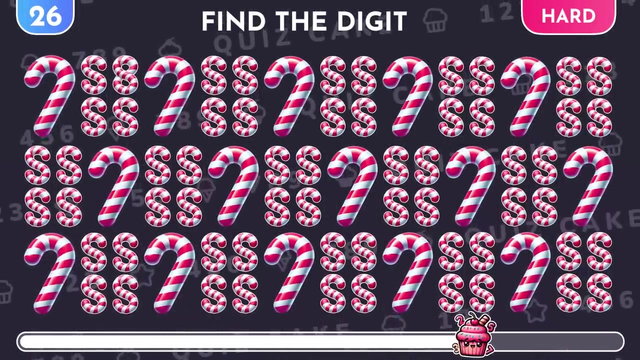 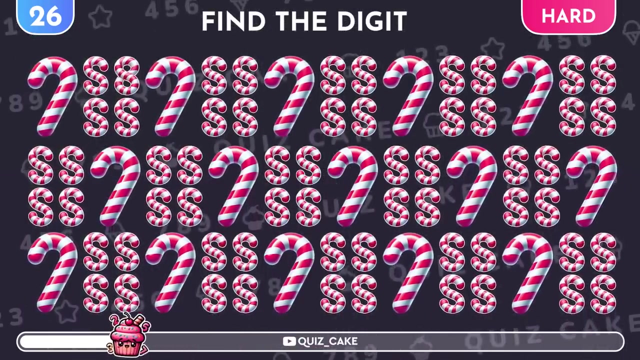 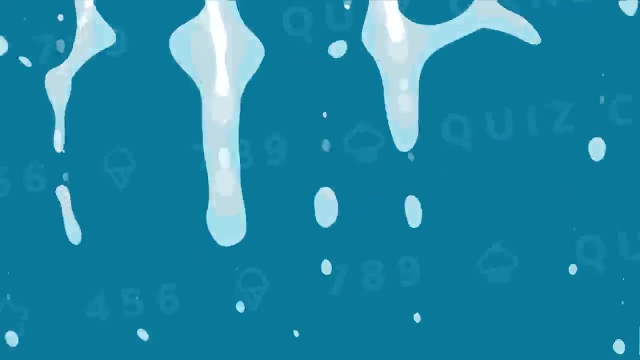 A traditional Christmas treat. Find the odd letter out. here It's the letter W- Awesome. Pay attention to the details here. Your task at this level is to find the digit. Wow, It's the number eight. Another test of your photographic memory. 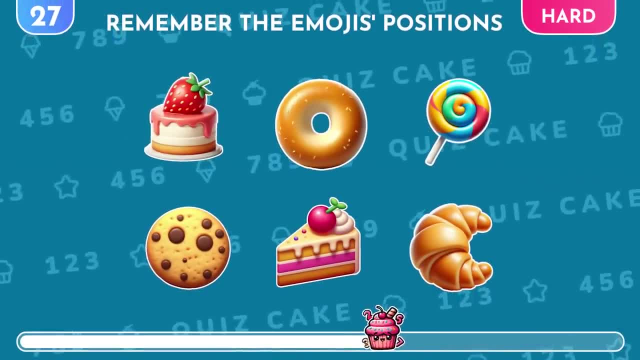 Remember the positions of all emojis? Oh, It's the number eight. Another test of your photographic memory. Remember the positions of all emojis? Oh, It's the number nine. Yay, Now recall where the lollipop was. Look at what you have found. 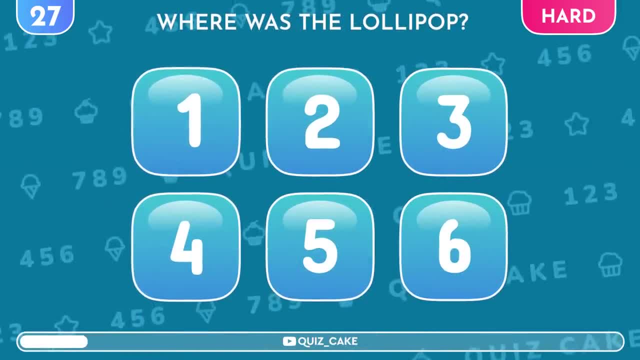 The first one is under the letter W, stereotypical. To find the digit, put the number in the middle of the paper. Then click the cursor on the bottom five. You will see the number seven. There it is. It's the number eight. 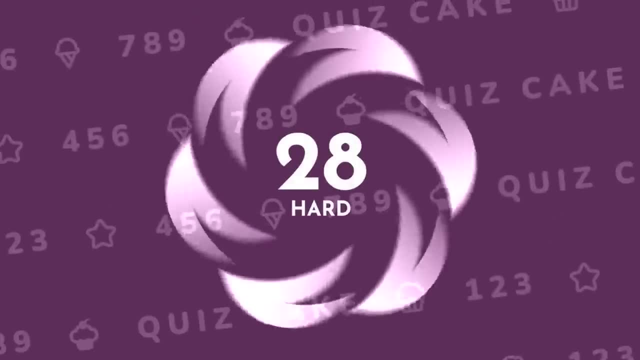 It's the dollop. Now, you have found the dollop. Now recall where the lollipop was. It's the dollar stamp, The number eight, It's the letter W. You've got it Next on our list. It's the birth of the doll.